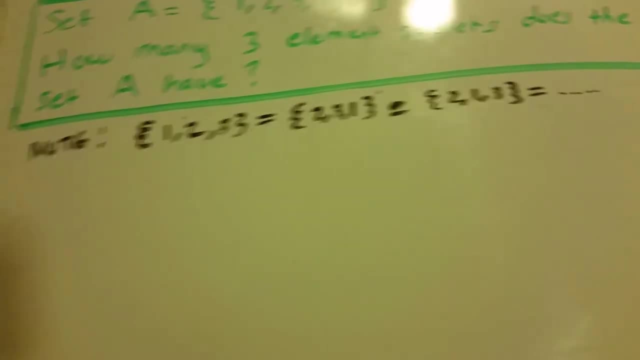 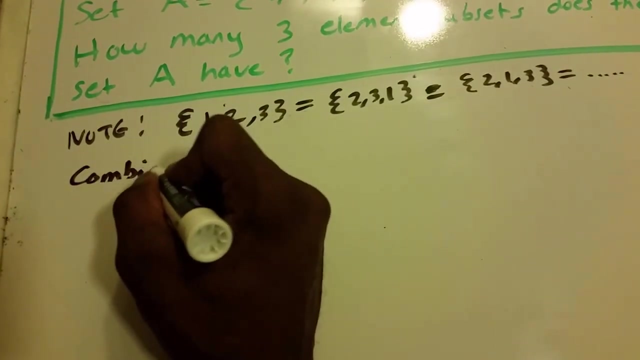 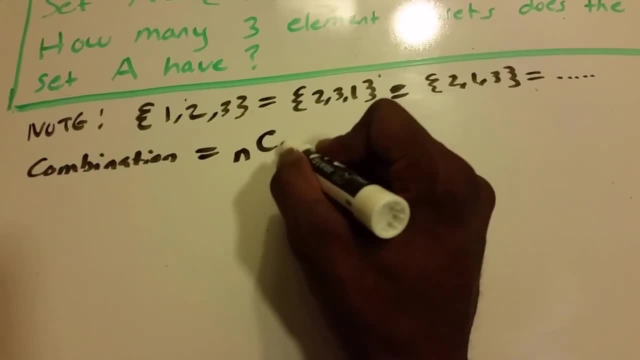 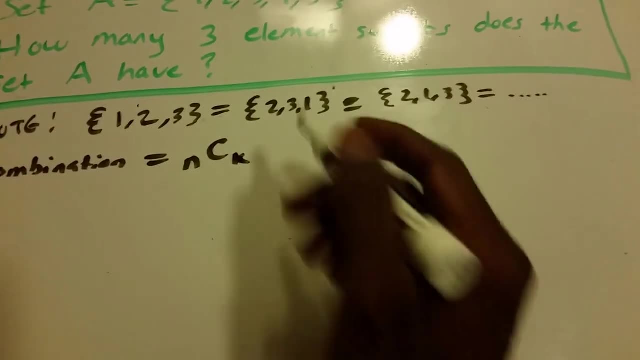 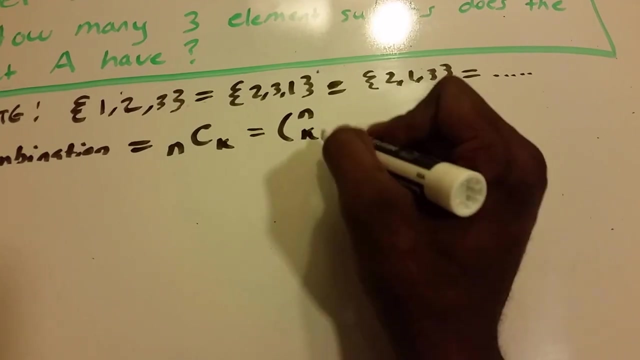 sometimes as a n, c, r, or you might even replace the r with a k, And then you also may see it look like this: We have n elements and we're choosing k of them, And then this is the actual formula. 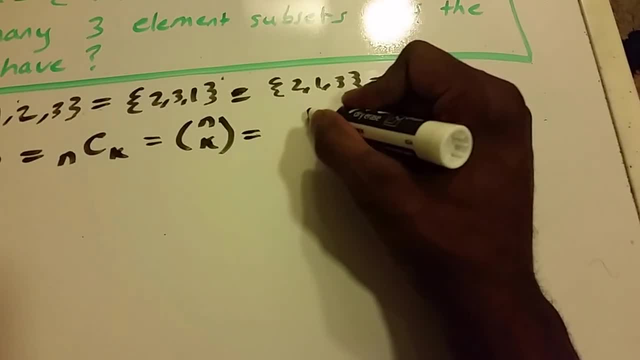 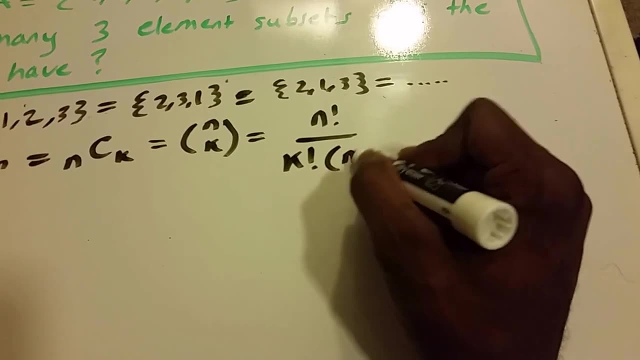 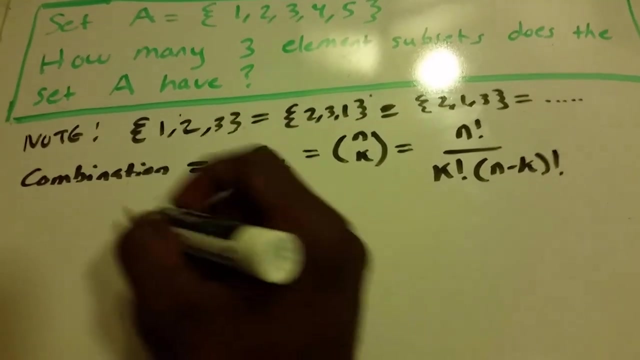 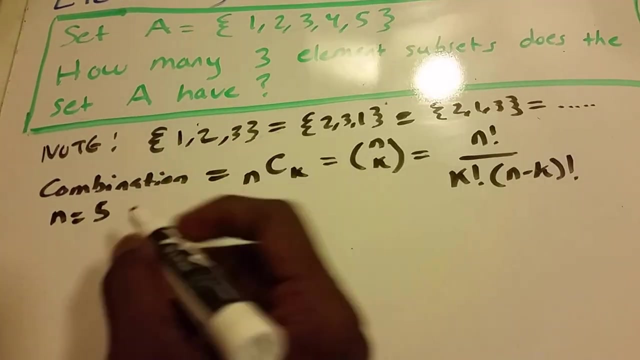 This is equal to n factorial divided by k factorial times, n minus k factorial. Okay, so what is our n value? Our n is equal to 5, because we have 5 elements in this set: 1,, 2,, 3,, 4, and 5.. And our k value is 3, because you want to know. 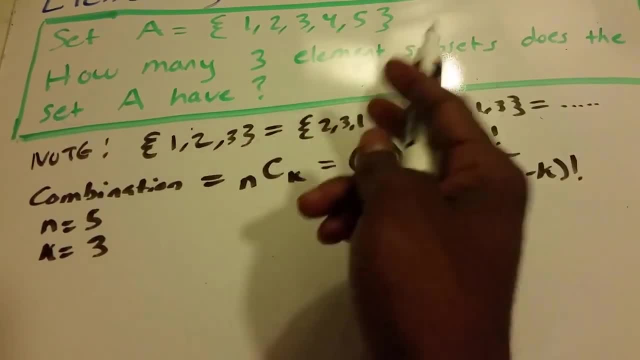 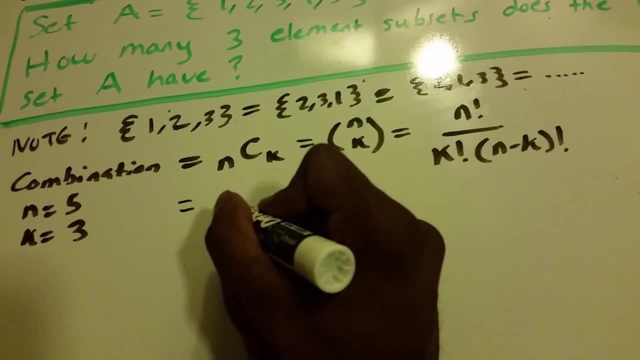 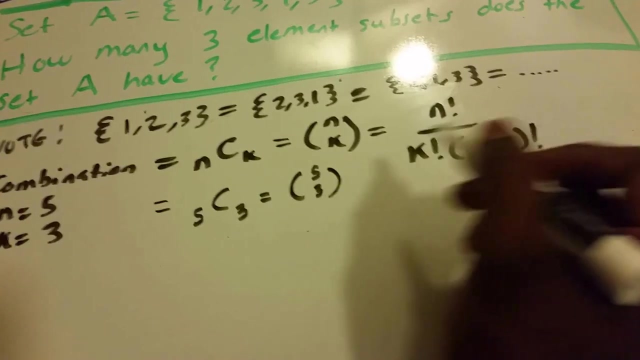 we want to get the number of 3-element subsets. So what that means. we plug this into our formula. here We get 5c3, which is equal to. well, we have 5 elements. We're choosing 3 of them. 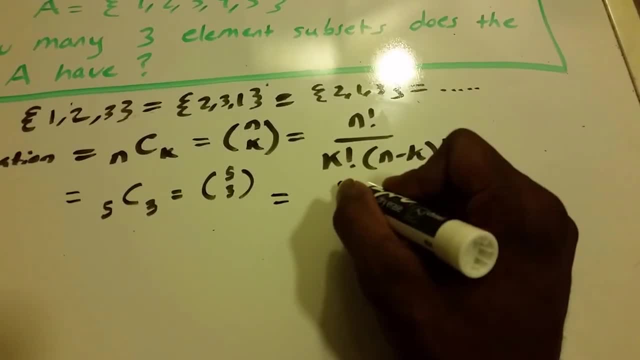 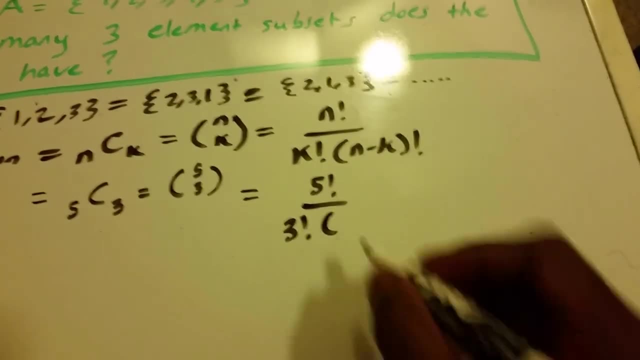 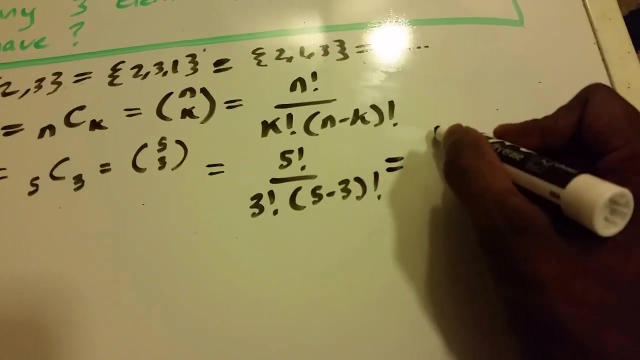 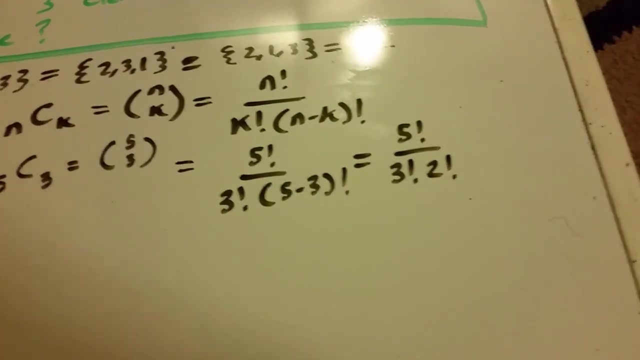 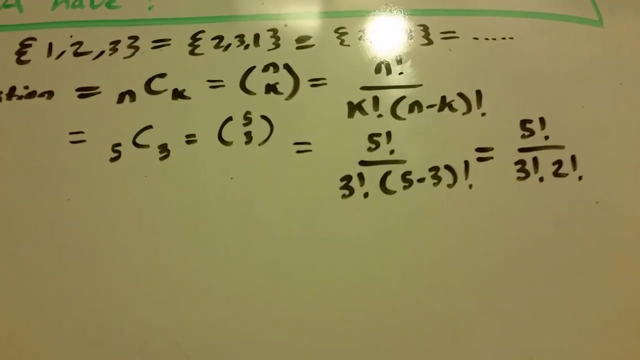 And this is equal to 5 factorial over 3 factorial times 5 minus 3 factorial. So now this is equal to 5 factorial divided by 3 factorial times 2 factorial. Okay, and I'm going to continue here down. Actually, I'll just go ahead and erase this. 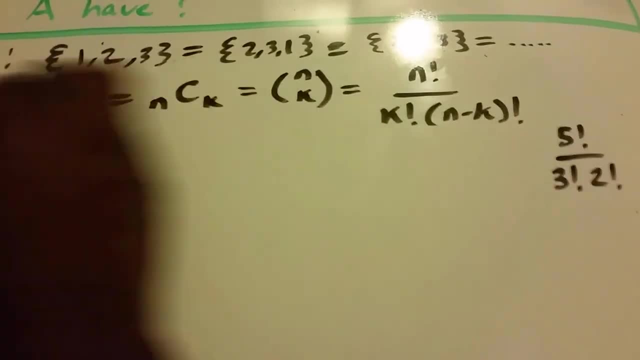 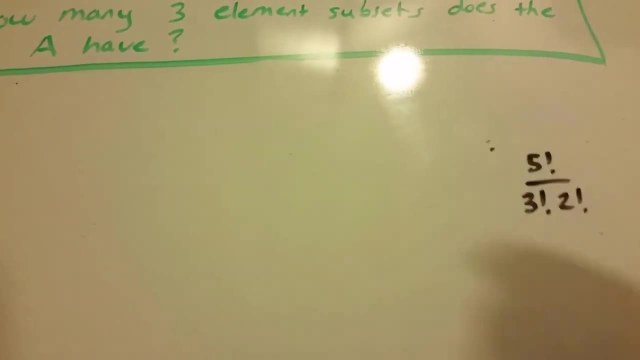 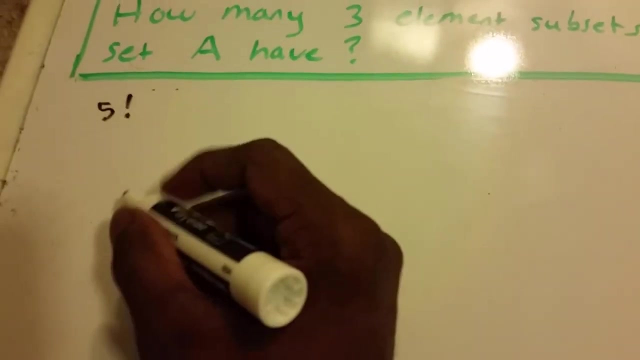 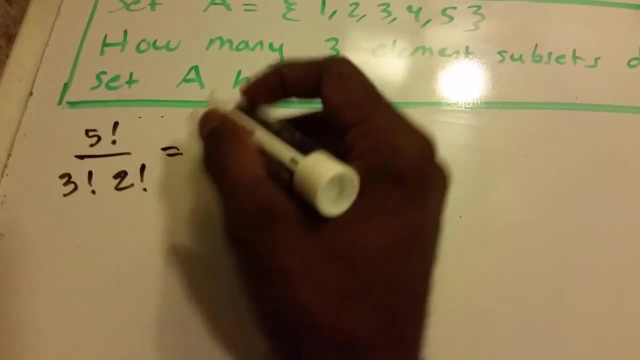 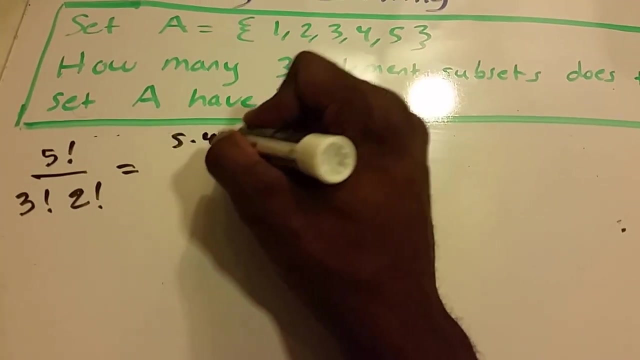 and keep that last solution. we have 5 factorial. So when we write that over here, we have 5 factorial divided by 3 factorial times 2 factorial. This is equal to 5 times 3, sorry, 5 times 4 times 3 times 2 times 1 divided. 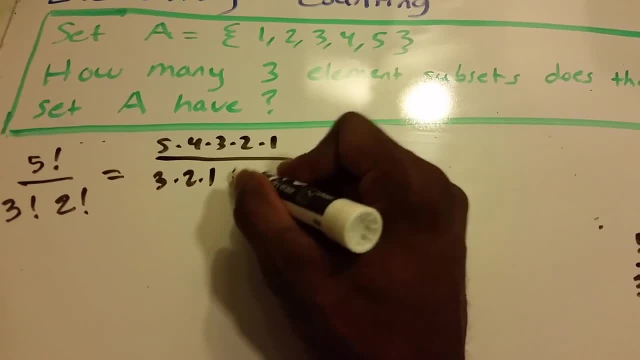 by 3 times, 2 times 1 times 2 times 1.. Go ahead andbeit ang, I will fought all of this and gloves me now right. Here is our method. We only need 5 factorial elements. When this time wetter and there is no Right, but we 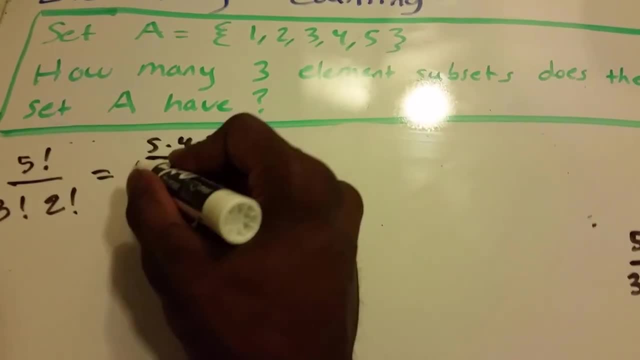 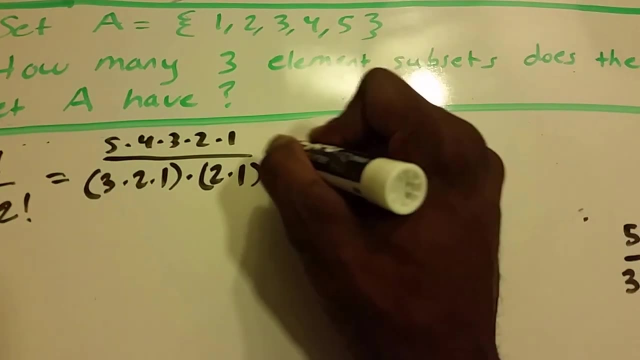 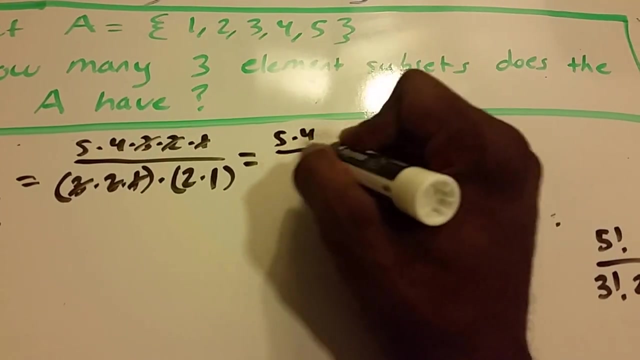 already knew we wanted to write another choice, So I'm going to write the thing Now. farmers can 1, okay, and so now what we can do is we can simplify this even more. just cross these out and we get 5 times 4, divided by 2 times 1, which is equal to 20. 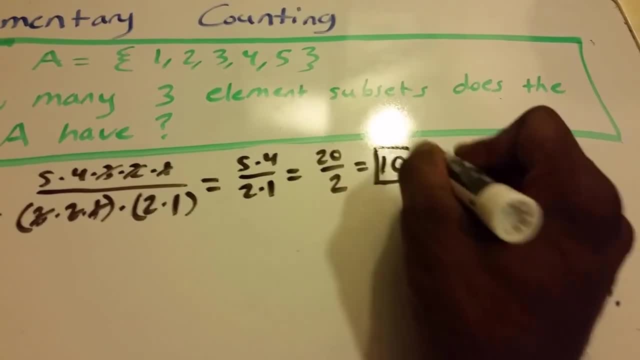 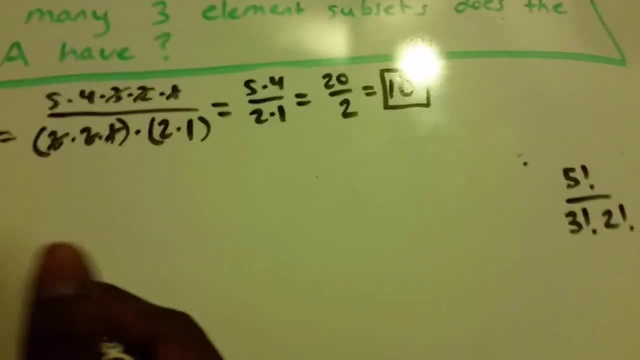 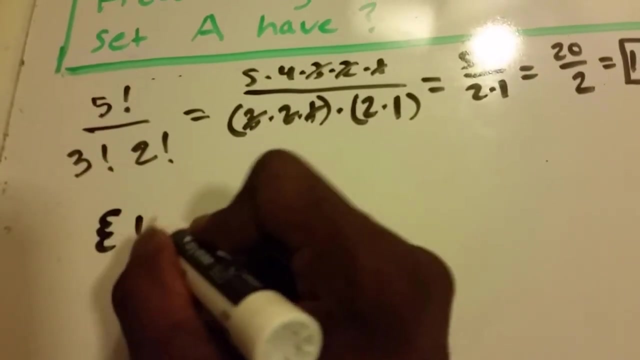 divided by 2, which equals 10. so our answer is 10. so let's check this, let's see if we can get 10 3 element subsets. so I'm gonna try to write them out here. so we get 1, 2 & 3, because that's in the set a, and we're getting 3 element. 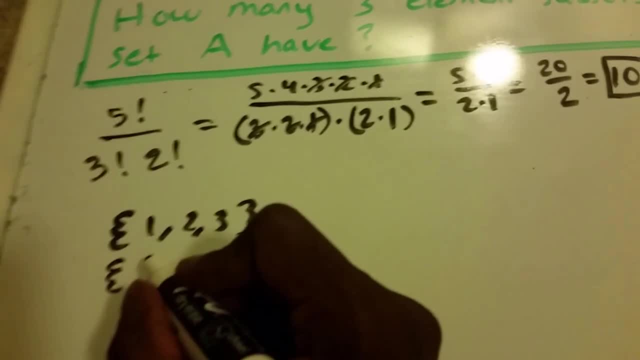 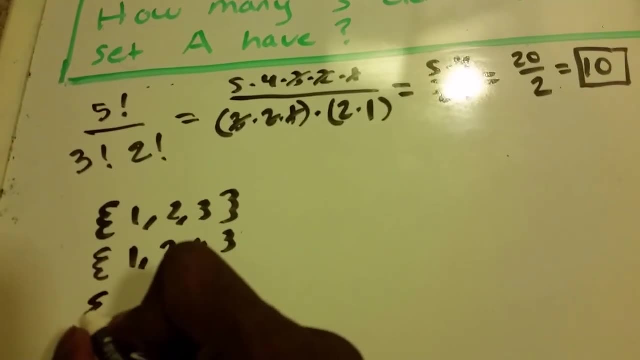 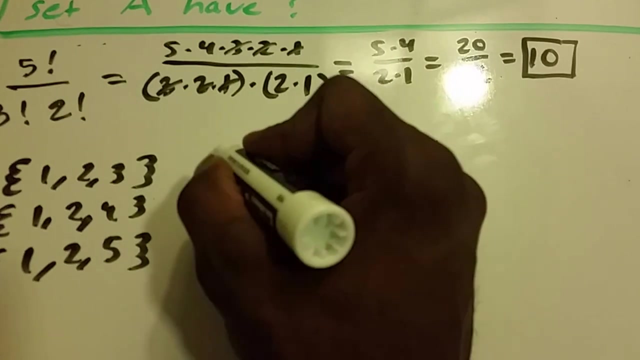 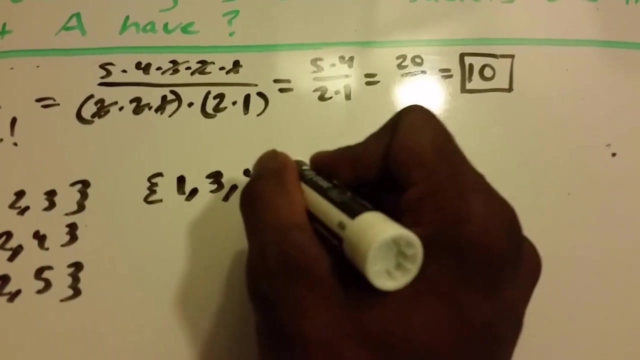 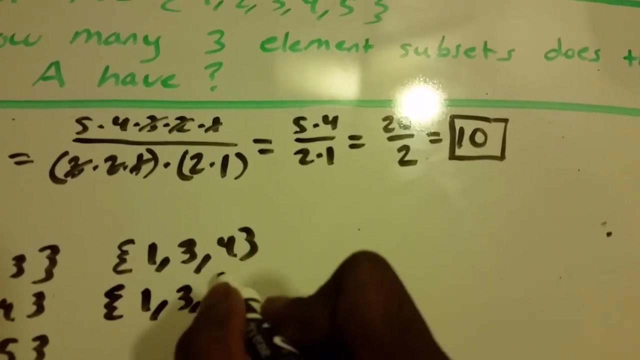 subsets next, I'm gonna do 24, okay, and 1, 2, 5, all righty, and let's keep going here. now we get 1, 3, 4, okay, and we're gonna do one, three, five, so right now. and we're gonna do 1, 3, 5, so right now. 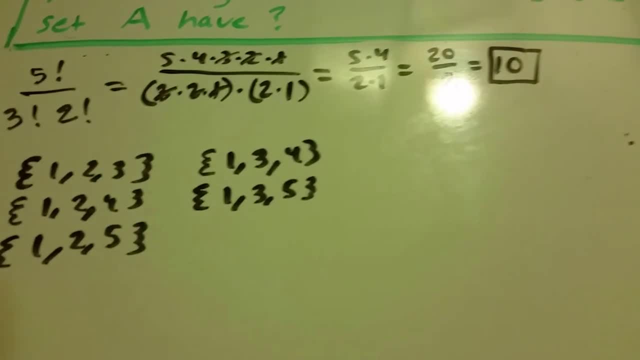 we got 9- 4, so we gotta get all of the terms there, specifically because we we got 9, 3, 4, so we, our гл… we lose all your slots이줄 in all our resumes that have five of these three elements, subsets and, according to our answer, we 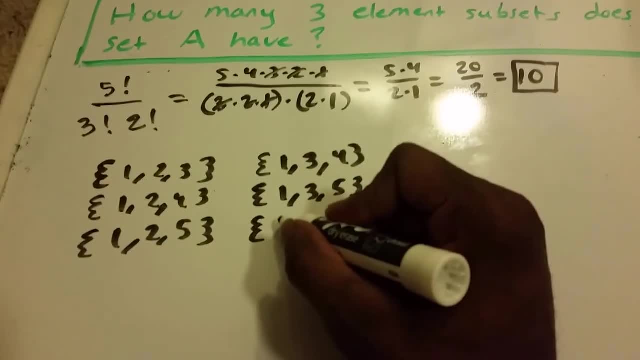 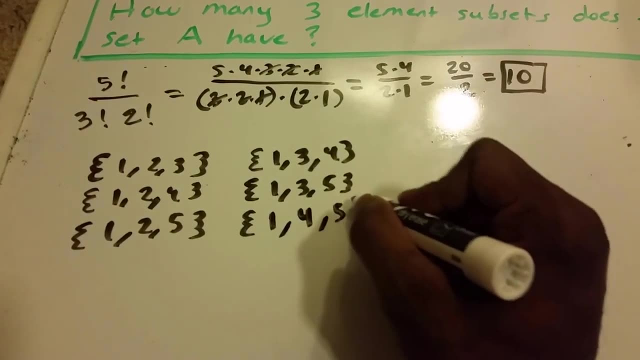 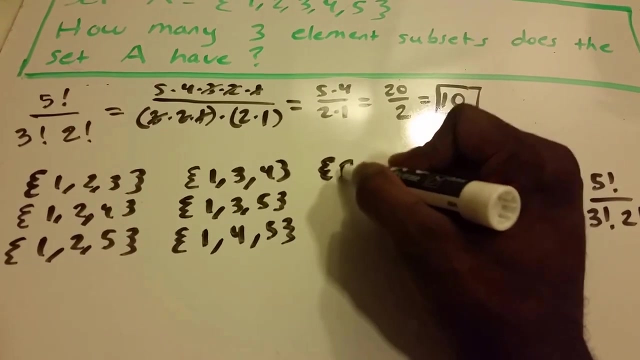 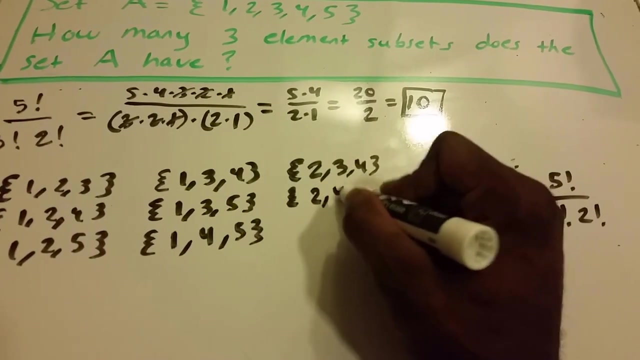 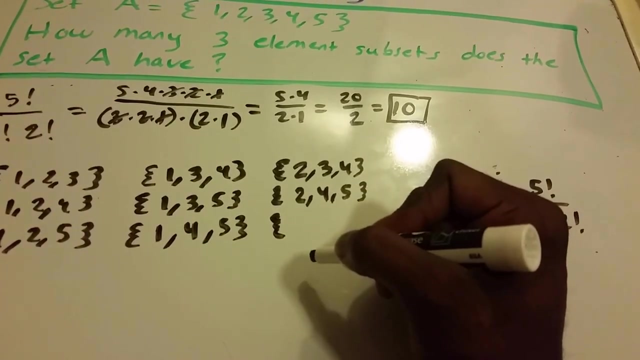 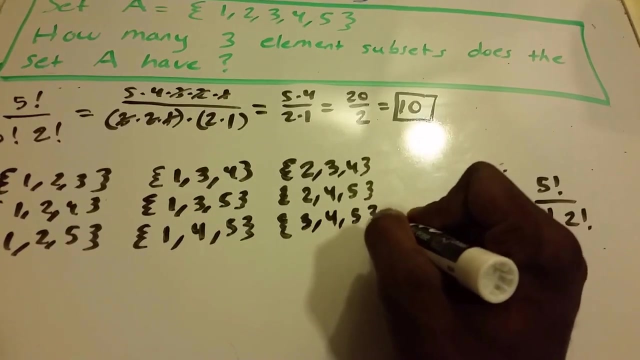 can get ten, so let's try next. one, four and five, and let's continue here. looks like we're done with the ones. two, three and four makes them get two, four and five. we can get three, four and five, so we got nine and now we just need to find. 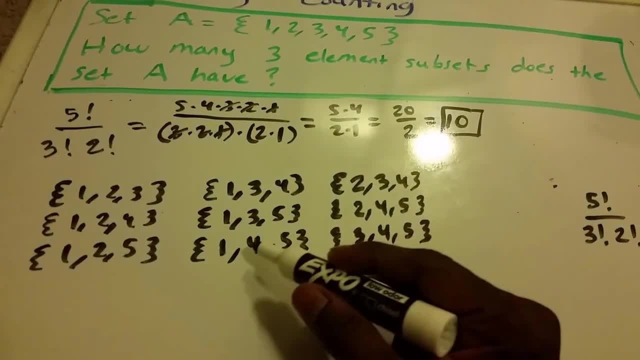 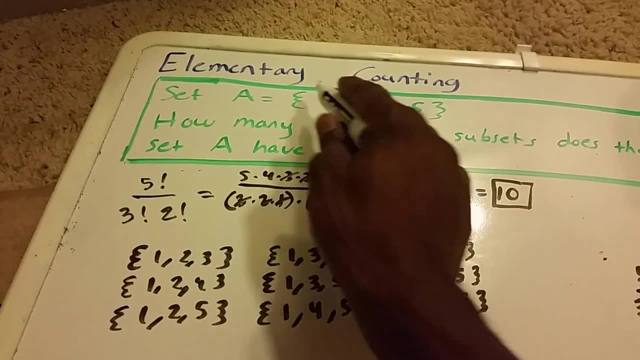 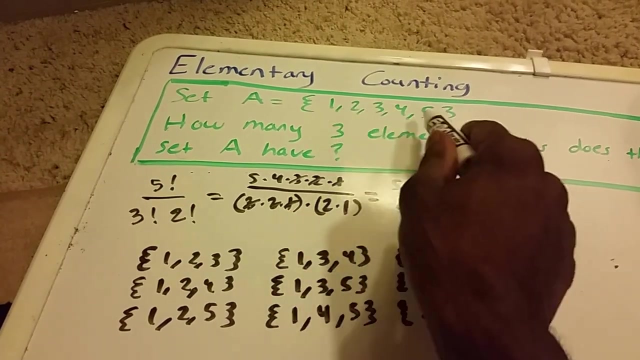 that last one. we have one. Let's check this. We have 1, 2, 3, 1, 2, 4, 1, 2, 5.. We have 1, 3, 4, 1, 3, 5, and that's all of our 1s. 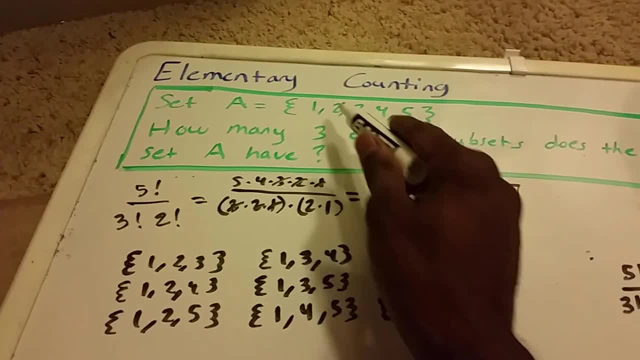 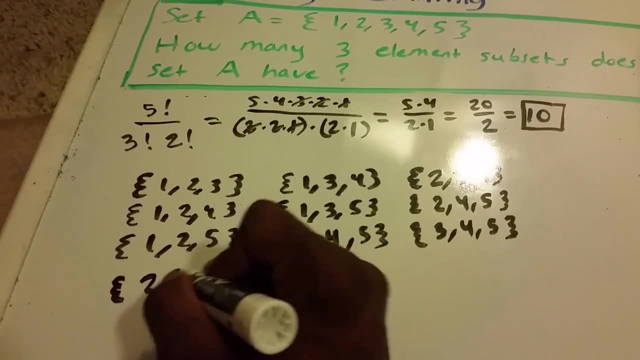 So we go to 2, let's check 2, 3, 4,. 2, 3, 5.. We do not have 2, 3, 5, and that's where it's at. So the last one is 2,, 3,, 5, and that's all 10.. 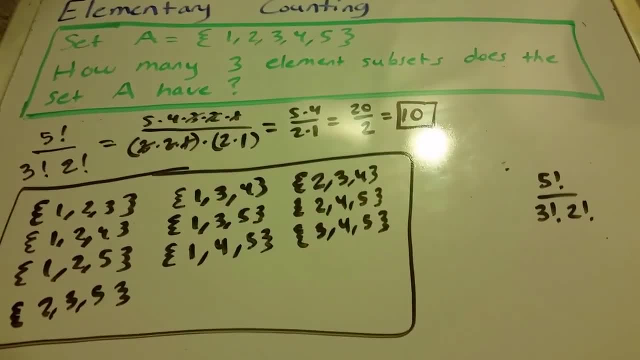 So thank you guys. I hope you enjoyed this video and I'll see you guys in the next video. 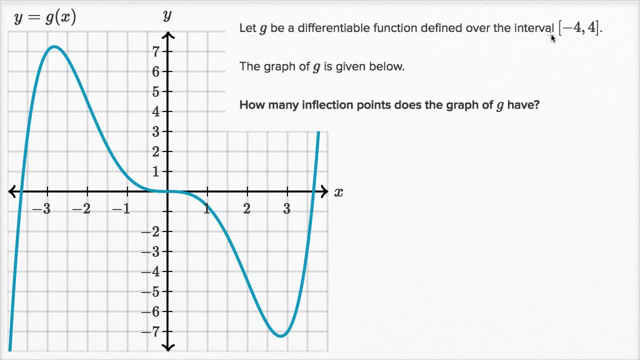 We're told. let g be a differentiable function defined over the closed interval from negative four to four. The graph of g is given right over here. given below, How many inflection points does the graph of g have? And so let's just remind ourselves. 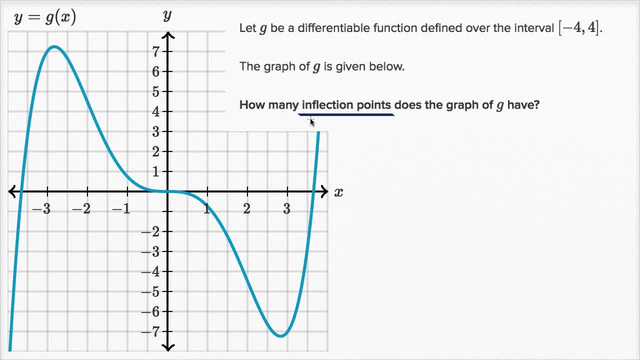 what are inflection points? So inflection points are where we change concavity. So we go from concave concave upwards, upwards. Actually, let me just draw it graphically- We're going from concave upwards to concave downwards. 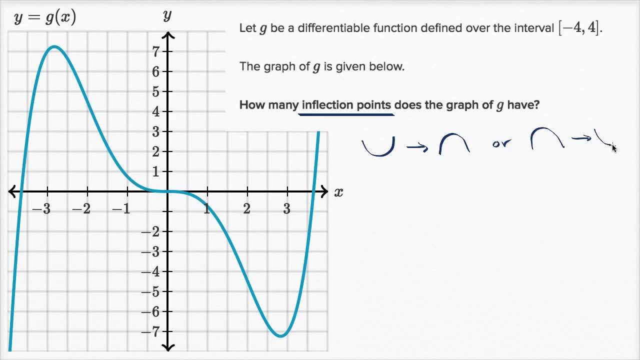 or concave downwards to concave upwards. So, or another way you could think about it. you could say: we're going from our slope increasing, increasing, increasing to our slope decreasing to our slope decreasing, Or the other way around.